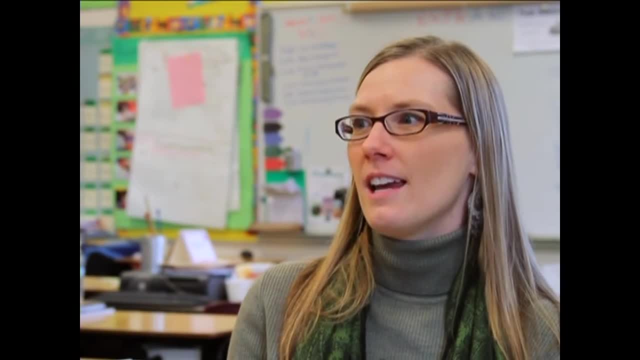 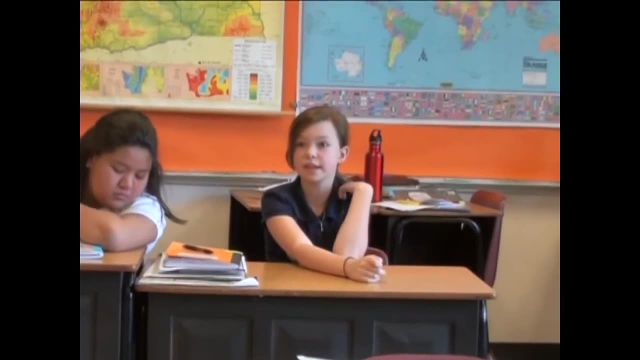 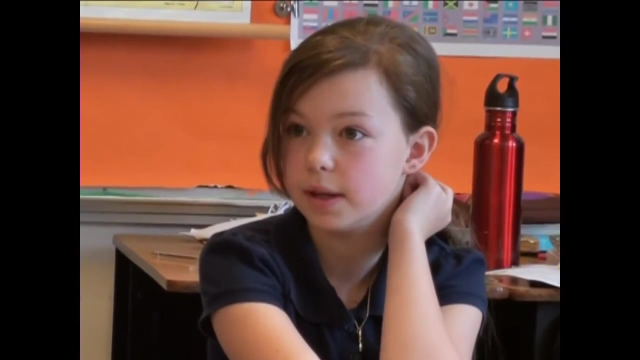 So I was pleasantly surprised to have them come in and engage students and you know, thinking about life and questions about life, But really I think that if you were, if you like for real, were going to die, I think you'd give up that and just take like what really really means. 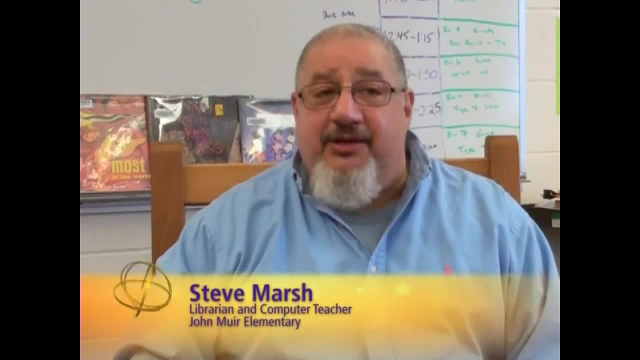 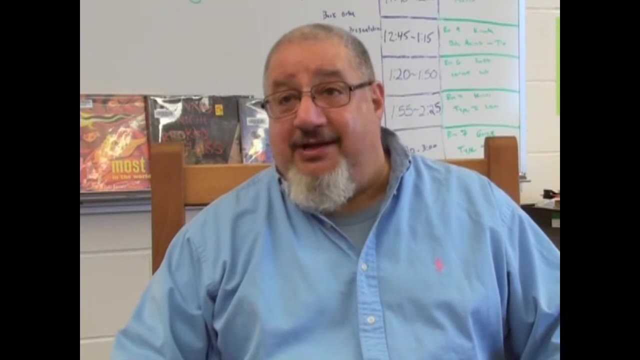 The kids are, like you know, raising their hands and they're barely containing themselves and they want to. you know we've had kids, just almost everybody in the entire class participates and wants to participate and is excited And it's just, it's wonderful to see. 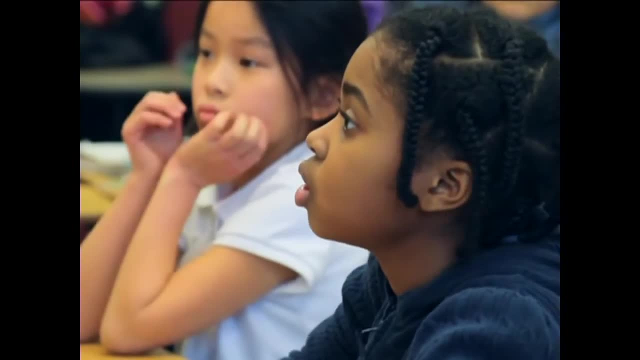 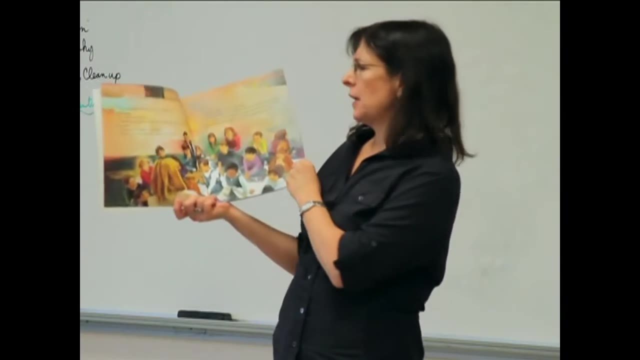 That's what I think really education is meant to do. In philosophy class, students explore their own thoughts, learning to think critically and creatively. What else could a contest be For this age? group sessions start with reading a story. 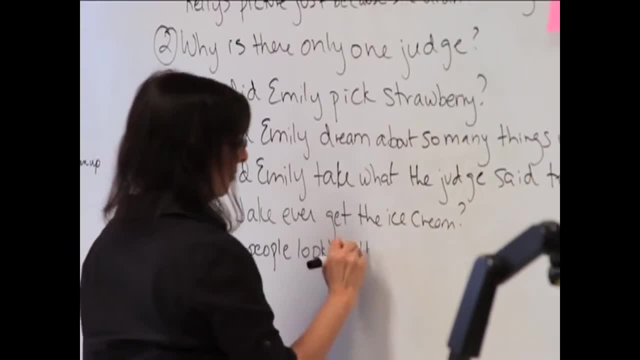 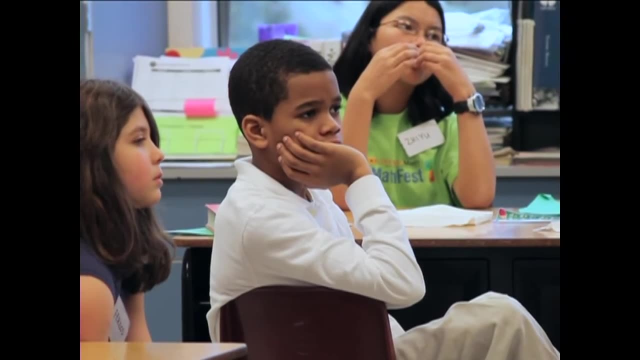 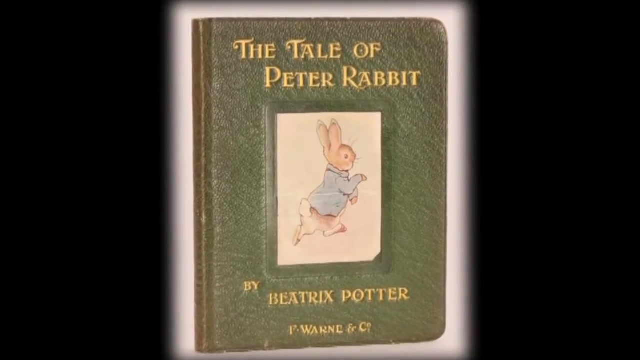 Next is coming up with questions and exploring possible answers. We're looking at the things that happen in the story and we're asking higher order thinking level questions, Kind of like the rabbit in the story who steals the stuff from Mr McGregor with his carrot patch. 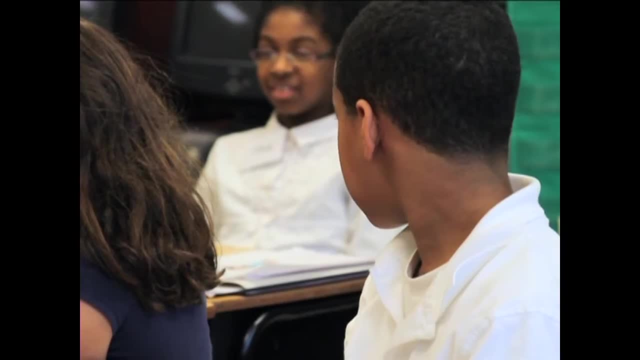 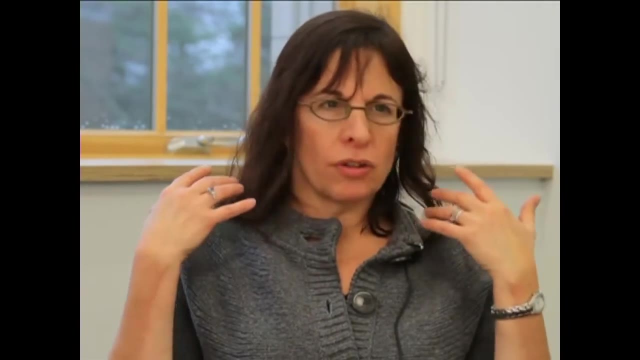 Could he control that? Was that wrong? Was it right? What if he was hungry? What if he was doing it to feed his family? Genuine learning takes place when you are not sort of passive recipients of knowledge you know being given to you. 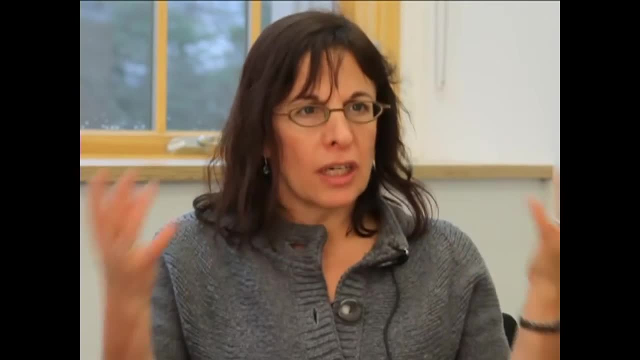 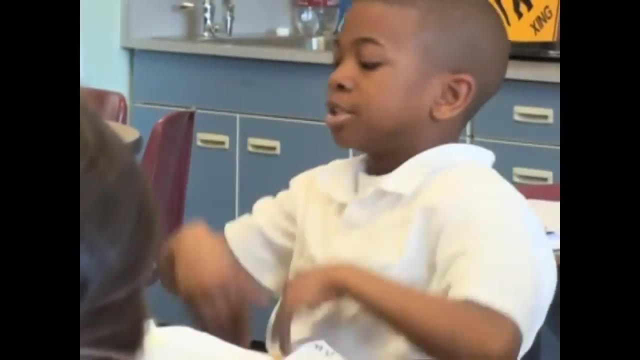 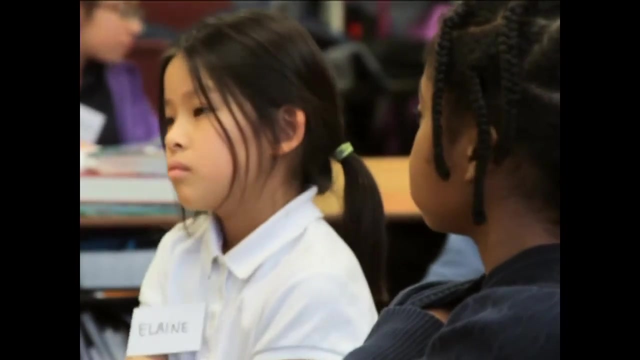 but are personally engaged in whatever it is. the topic is in the classroom and a connection is made for you. It makes me like just think. While philosophy helps students cultivate reasoning and analytical skills, it also fosters an appreciation for other people's viewpoints. 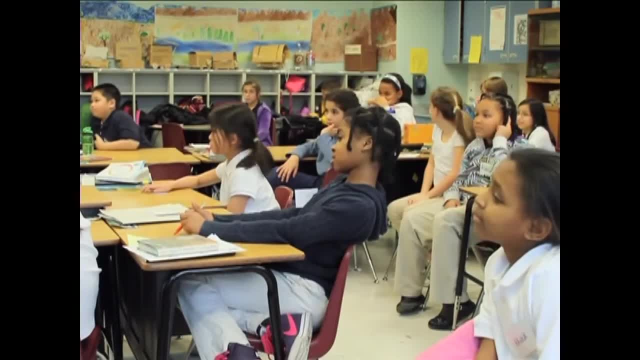 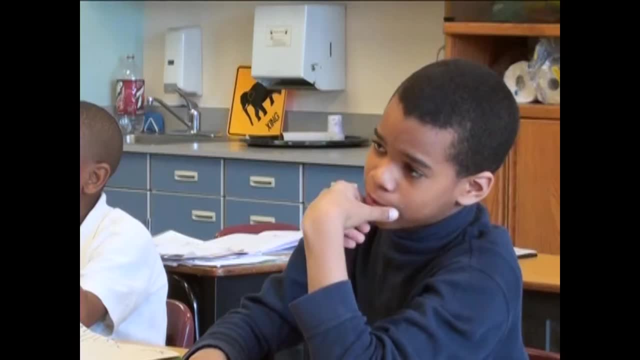 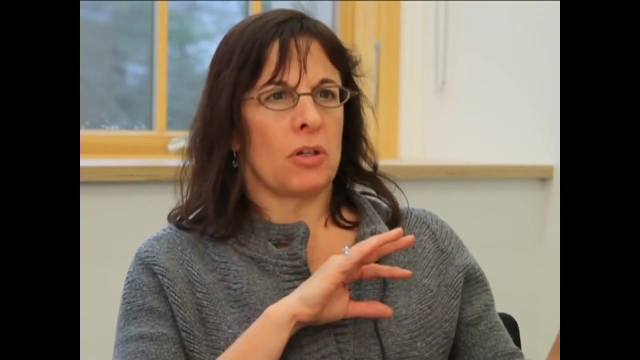 And that may be the best lesson of all- The participants start to recognize that there are a whole range of perspectives from which the world can be viewed, and that those perspectives can be very different from your own, but they don't have to then be threatening.